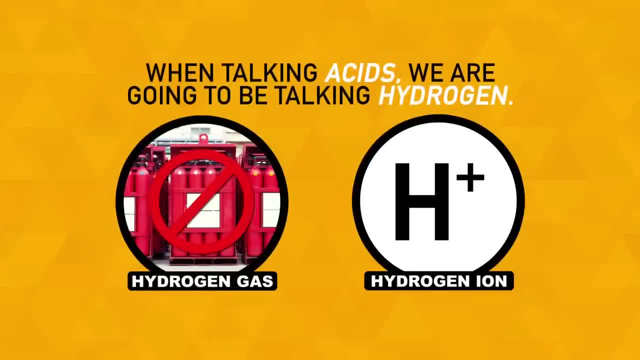 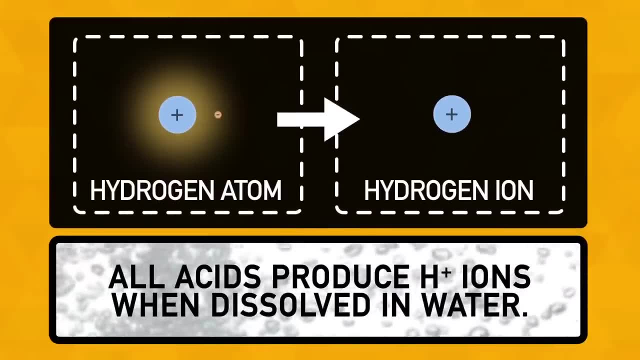 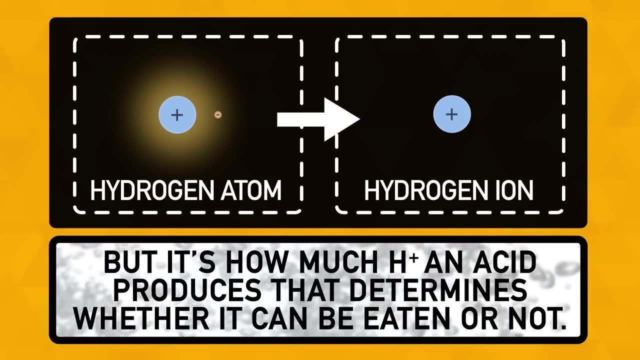 When talking acids, we're going to be talking hydrogen. Not the gas, but rather the hydrogen ion H+. This is a hydrogen atom that has lost its one and only electron. All acids produce H-plus ions when dissolved in water, but it's how much H+, a specific acid can produce in water that will determine whether it can be safely eaten or not. 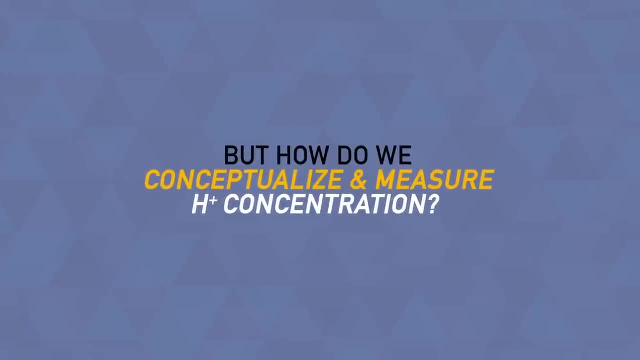 But how do we conceptualize and measure H-plus concentration? Soren Sorensen, a Danish chemist, pondered this question when he worked at the laboratories of a commercial brewery in Copenhagen. 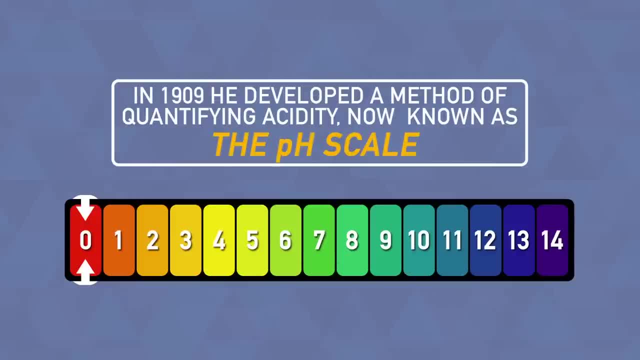 It was in 1909 that he developed a method of quantifying acidity, what is now known as the pH scale. His scale works by simply converting the concentration of hydrogen ions 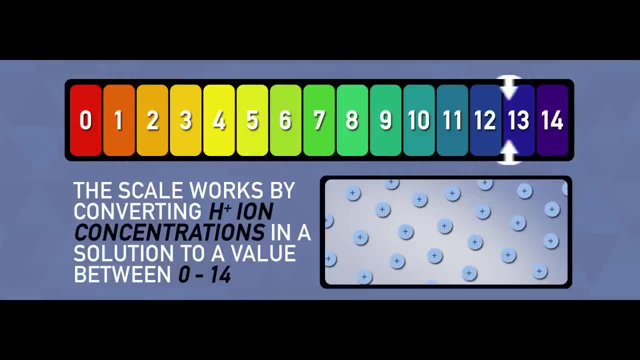 in a solution to a number between 0 and 14. If a chemical is acidic, then its pH will always be below 0. 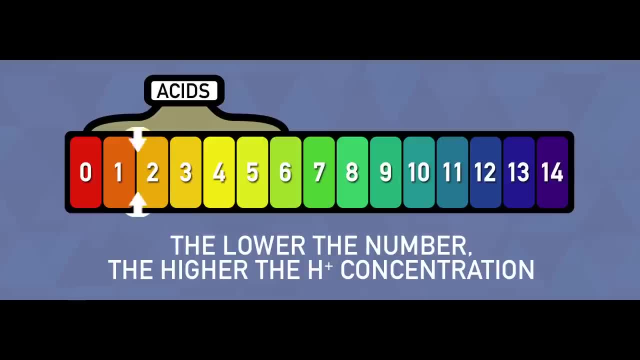 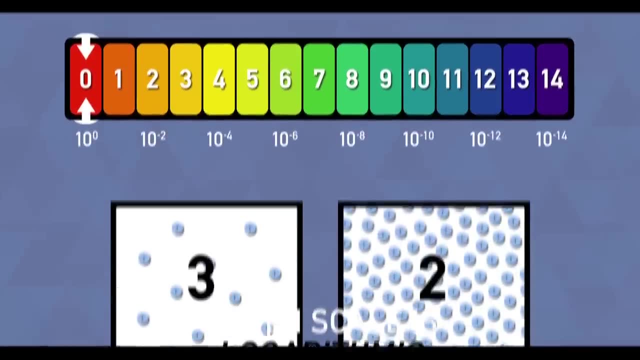 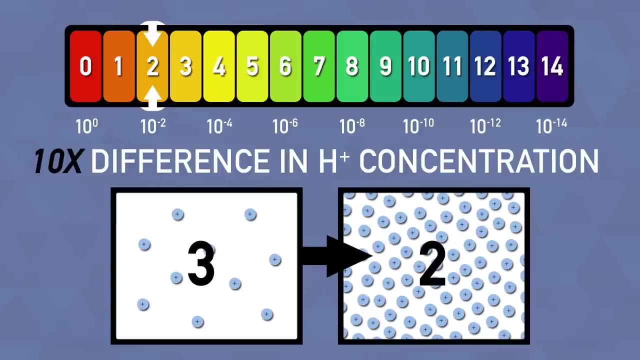 The lower the number, the higher the hydrogen ion concentration. The pH scale is a logarithmic one, meaning that one unit difference on the scale, say from 3 to 2, means a ten-fold difference in H-plus concentration. But 0 to 7 is only half of the picture. So what about all these numbers above 7? Substances that correspond with this 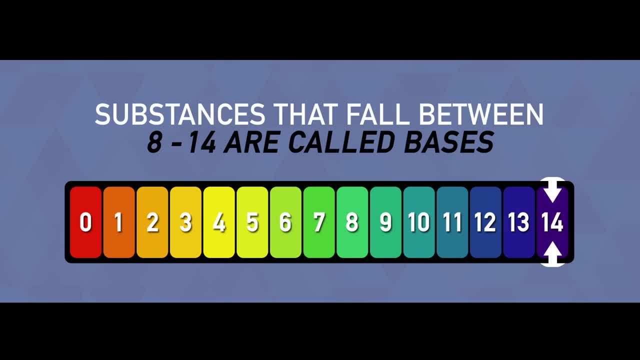 half of the scale are called bases, and they are the chemical opposites of acids. The 7 on the scale represents neutral pH, what would be perfectly pure water. 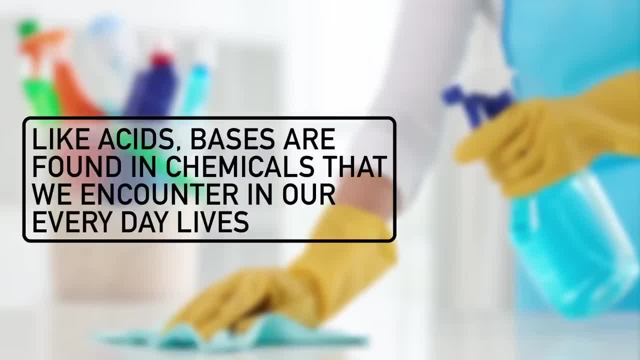 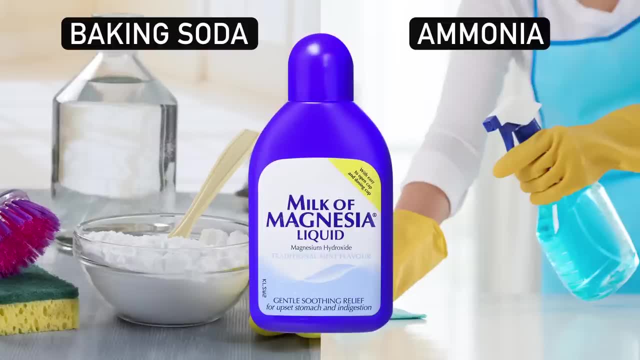 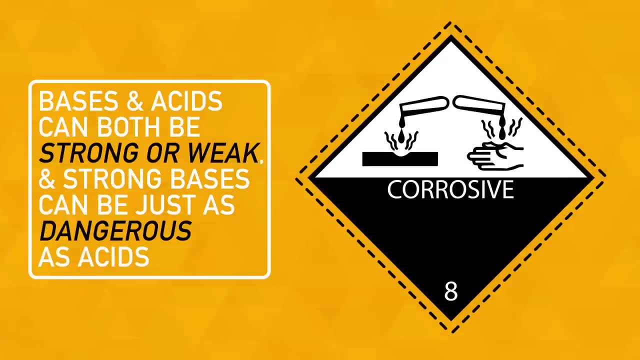 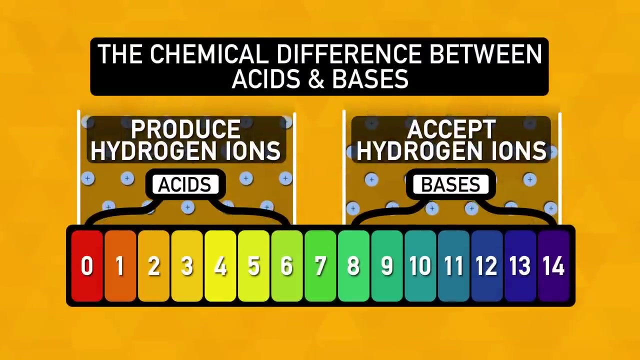 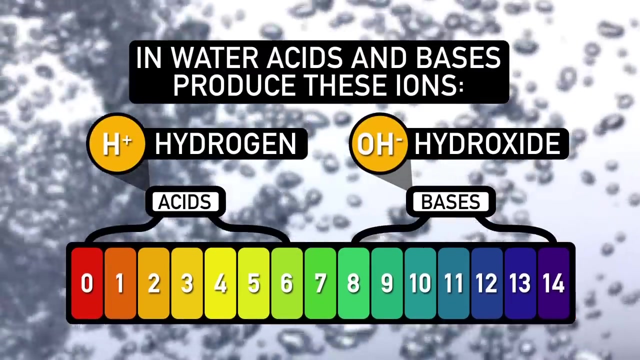 Like acids, bases are found in chemicals that we encounter in our everyday lives, cleaning products such as ammonia and baking soda are bases, as are some simple medicines such as milk and magnesium. They're bitter to the taste, and often slippery to the touch, like soap. Even though bases are different than acids, they too can be strong or weak, and a strong base can be just as dangerous and corrosive as a strong acid. Chemically, the difference between acids and bases is that acids produce hydrogen ions and bases accept them. In water, acids produce a neutral salt. So, for instance, water is the most capable acid to produce oxygen ions for a certain period of time. But this indicates that acids are H plus ions and bases produce OH negative ions. 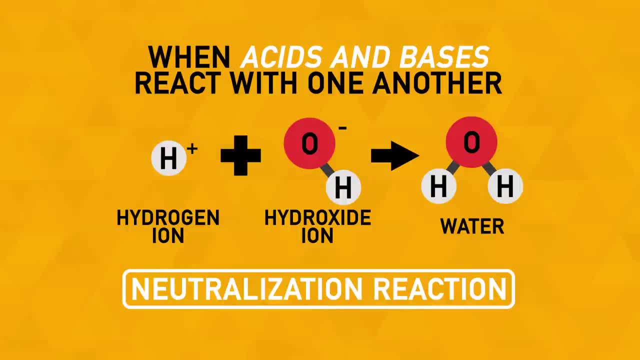 In reactions between acids and bases, hydrogen ions will react with hydroxide ions to make water. 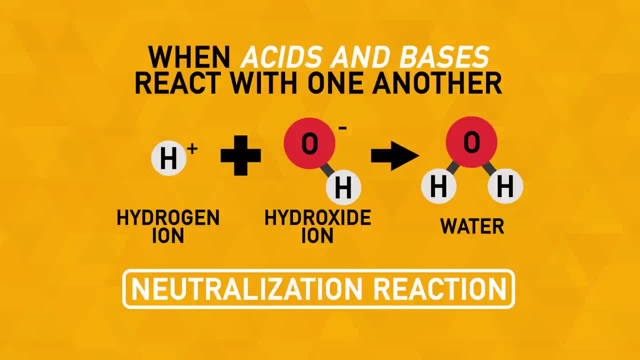 This type of chemical reaction is called a neutralization reaction. 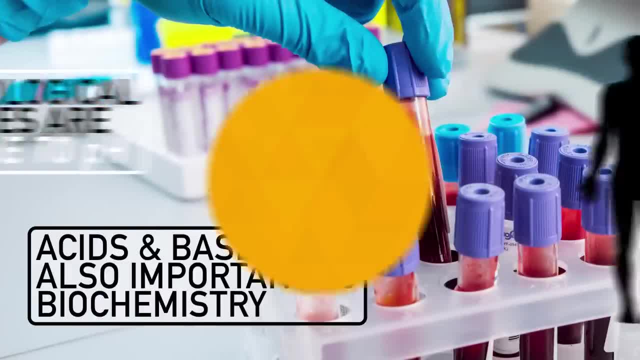 Acids and bases are also very important in biochemistry. Many biological processes are sensitive to the pH of the surroundings, so controlling acidity in the body is crucial.